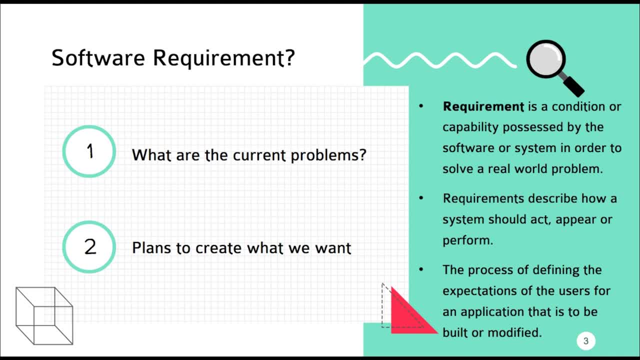 First of all, I am going to talk about people working with software technology each day, roasted with software to injured, For example, a software engineer like an autor service engineer for a private company. world problem Requirements describe how a system should act, appear or perform. So 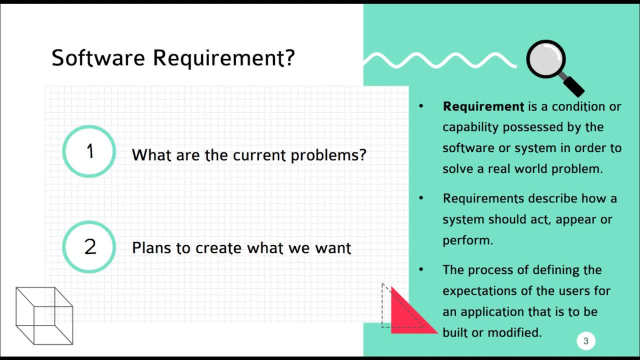 it's a process of defining the expectation of the users for an application. When I say the process of defining the expectation of the users, we have to consider two points. Number one is what are the current problems, and point number two how we are going to plan and solve the problems. So what is? 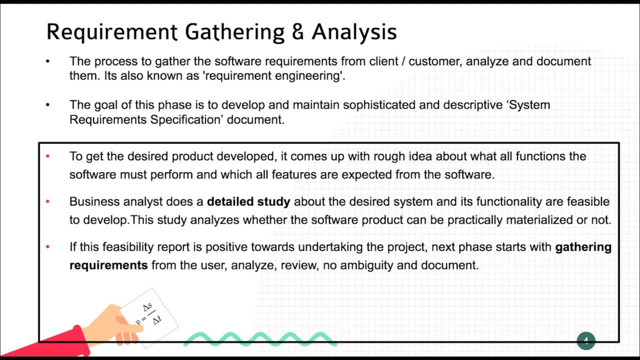 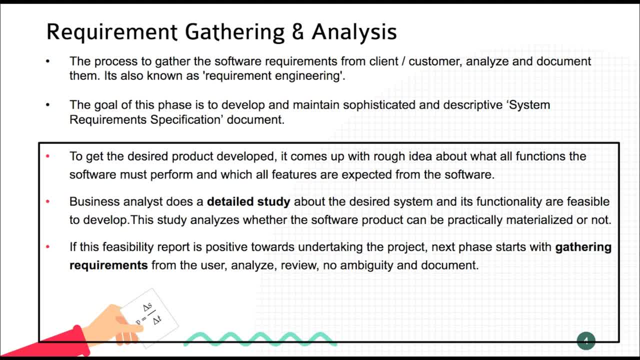 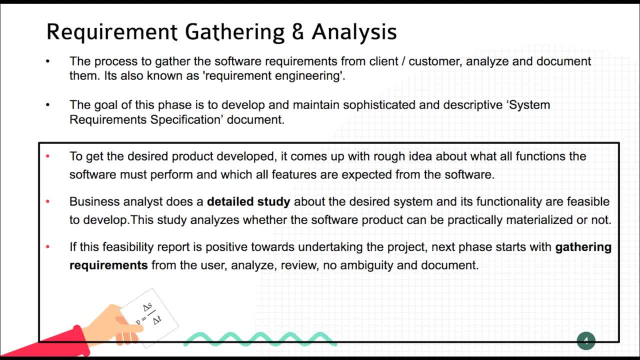 functions the software must perform and what are the features it must have. So it's all start with a rough idea and it's kind of a single line requirements. So business analyst does a detailed study about. So business analyst does a detailed study about the rough idea and the single line requirements. They collect the information. 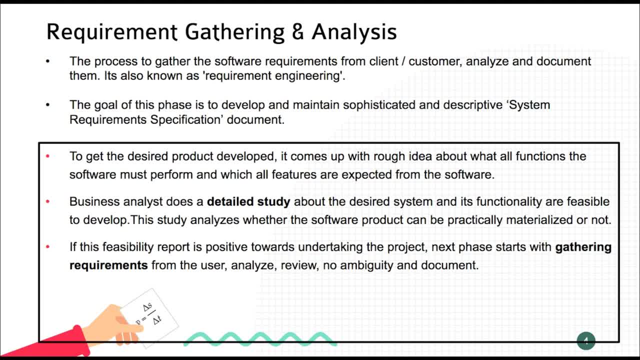 the rough idea and the single line requirements. They collect the information from the surveys and the SMEs and from the existing system functionalities. from the surveys and the SMEs and from the existing system functionalities. They will make a detailed study about it. So the output of the study it's going to 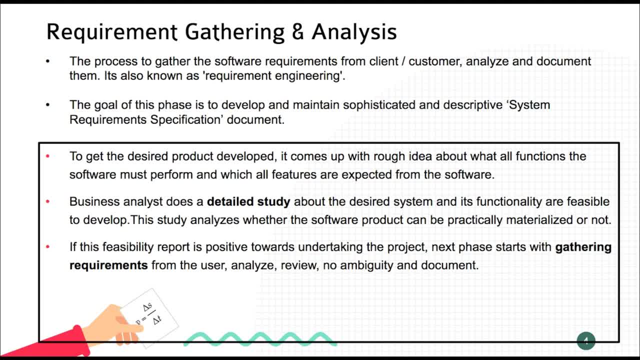 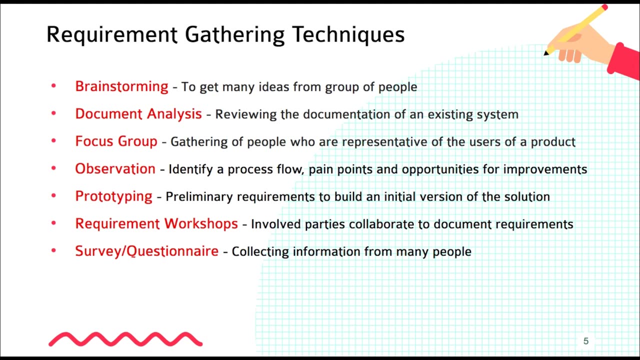 give us the result. If the report is very positive, then the next phase is gathering the. the next phase is gathering the requirements from the users, analyze them, review and make sure there is no duplicates, and document them for a further process. so these are the few techniques for gathering requirements. 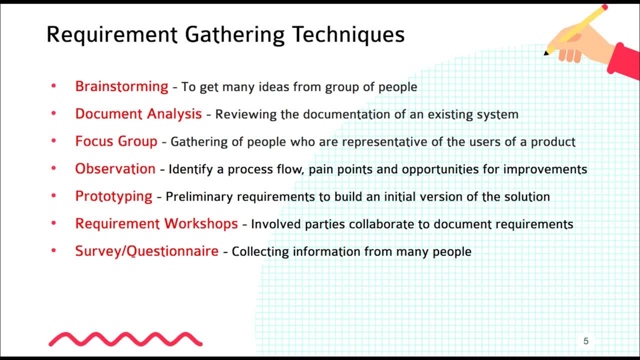 brainstorming so to get many ideas from different people. and document analysis- review the documents of an existing system and focus group observation: identify the whole process and what are the pain points and what are the improvements that we have to do. and prototyping it's a we have to get the very basic requirements or very important requirements, and 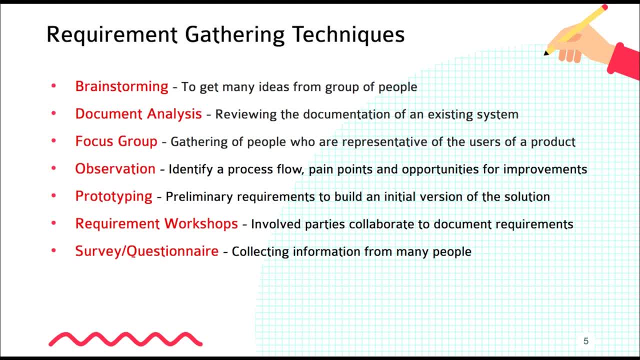 not the whole big requirements. we'll try to create a small version, initial version, of the solution and present it to the customer. and and conducting the different- uh, the requirement workshops- okay, involving multiple people- and document the requirements. and finally, there are other ways of doing it- uh, the survey and question or, you know, collecting the information. 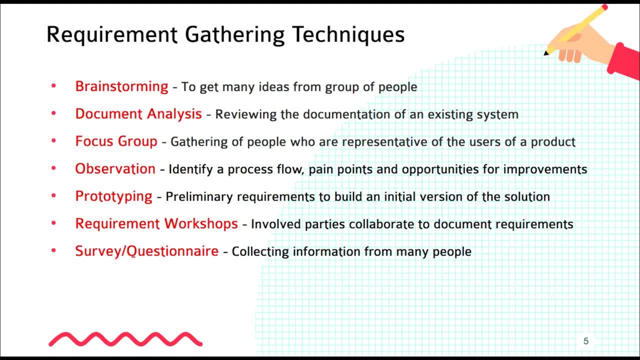 from the users, for example, the mobile phone or anything. so you might have seen a lot of surveys floating in the internet. where you have to. there would be questions on uh recent release of the mobile phone or what are the features that you are looking for? what is the good and bad that kind of a questionnaire or survey would. 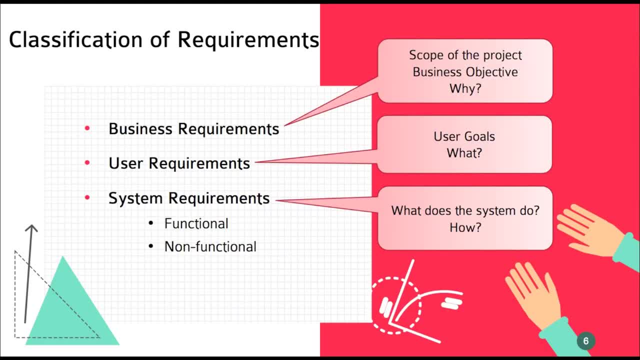 help us, to you know, gather the requirements. so let's talk about the classification of requirements. first and foremost is the requirement code. so when i say the requirements, it would be there are three types: business requirements, user equipments and system requirements, the. what is the business requirement? it's going to talk about the scope of the project. 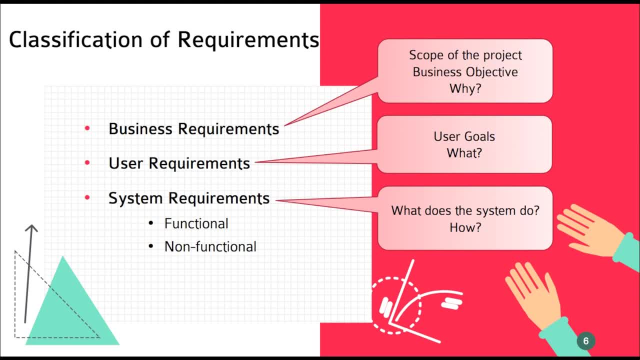 the objective. so why do we need this software? why do we need the system me? so, when it comes to the requirements, it's going to answer the question for what it's talking about- the user level goals and the system requirements is a very detailed one, and it's going to tell us how. what does the system do? and the system requirements. 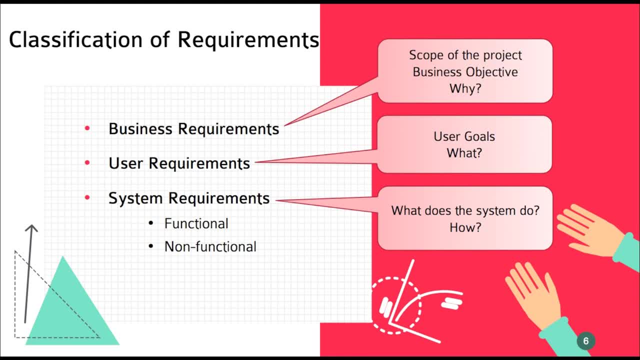 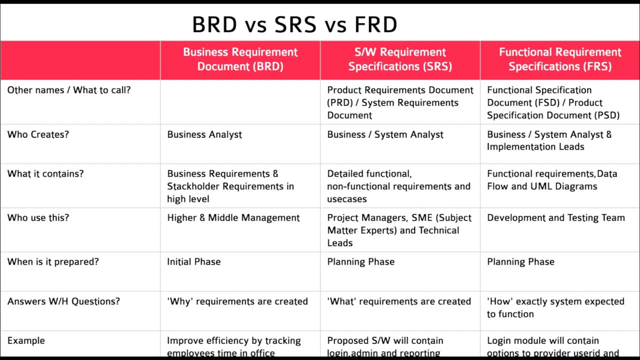 would be classified into two types of requirements. one is functional and non-functional. the functional is going to talk about what non-functional is going to talk about how. in this slide- it's a very, very important slide- it's going to talk about the difference between business requirement document. 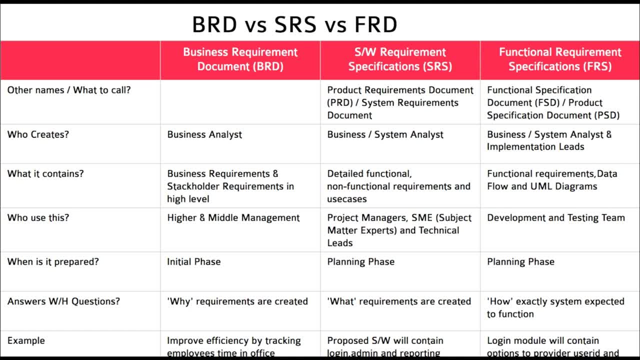 software specification and the functional requirement specifications. so I classified into seven points here. one is: what are the other names are referred for this document, the SRS, the software document specification. there is other name called the product requirements documents, the PRD and the functional requirements. they call it as a functional specification document, FSD or 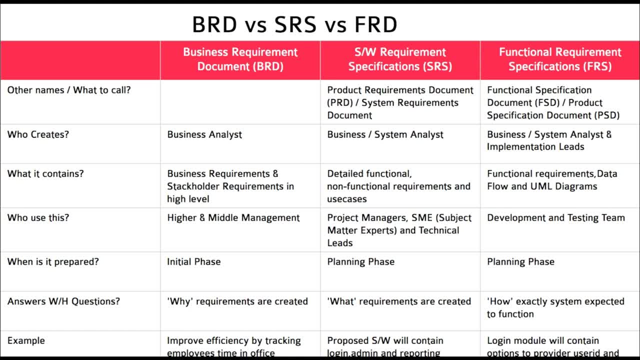 product specification document, the PSD. so who creates this documents? so BRD. the business requirements has been created by the business analyst. the SRS would be created by business and system analyst. and functional it would be created by the business system analyst and the implementation leads and what it. 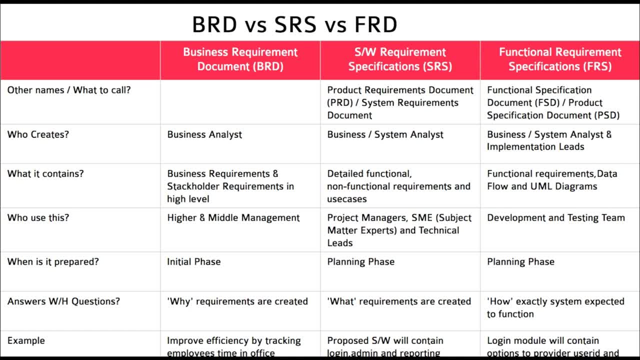 contains the BRD, contains the business requirements, the goal of the project, but the business requirements, the stakeholder requirements, in very, very high level. when it comes to SRS, it's a detailed level of functional and non-functional requirements and the use cases. when it comes to the functional, 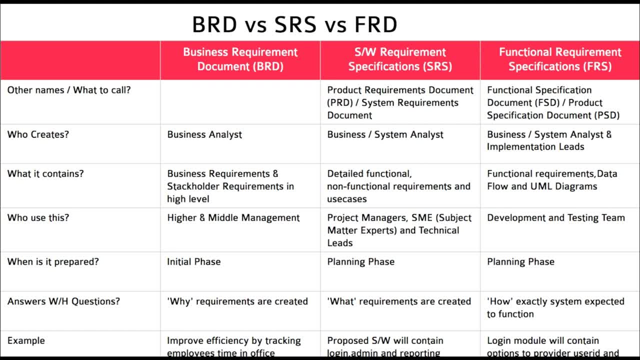 requirements. its contains the functional requirements, data flow and the UML diagram. who's going to use this? or documents the BRD? it would be referred by the higher and middle level management. the SRS would be referred by project managers, SMEs in the subject matter experts and technical. 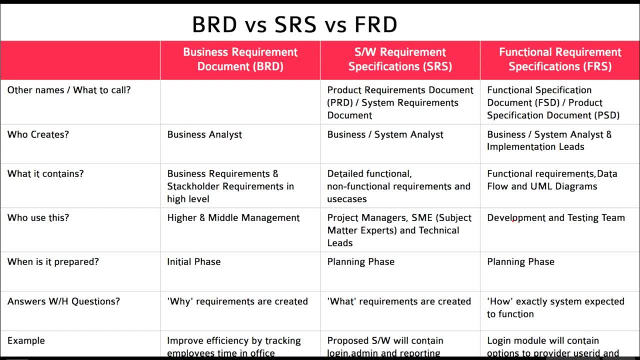 leads and functional. so that is going to be used by the development and testing team. so when it is prepared. so BRD is the initial one. it's prepared in the initial phase of the project. from there the SRS would be prepared during the planning phase and then the functional. so, as mentioned in the 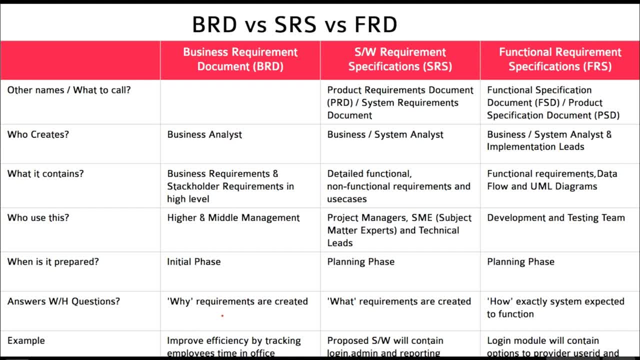 previous slide. BRD is going to talk about why requirements are created and SRS is going to talk about what requirements are created. Functional, it's going to talk about how exactly the system should perform. Here is an example. I mean there is a detailed use case I mentioned in the slide, but for 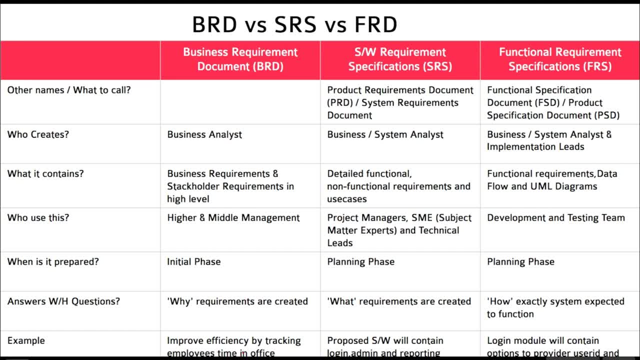 example here, the improve efficiency by tracking employees the time in the office. right, it's a business requirement. for the business requirement, what SRS is going to have is it's going to say the proposed software will contain the login, admin and reporting page. when it comes to functional, it's going to say: 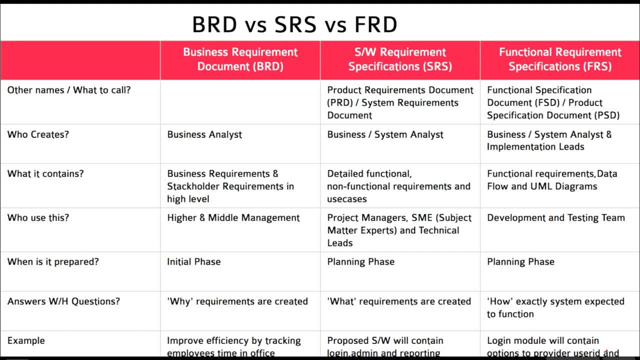 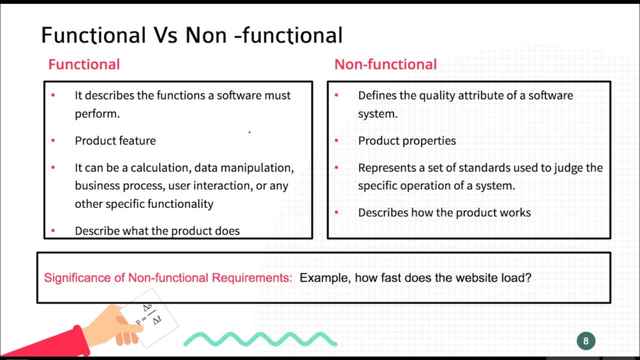 the login module will contain options to provide user ID and the password. so here we are going to see what is the difference between functional and non-functional requirements and what is the significance of using non-functional requirements. so the functional requirement is going to talk about what that means. it's going to describe the functions your software must perform. 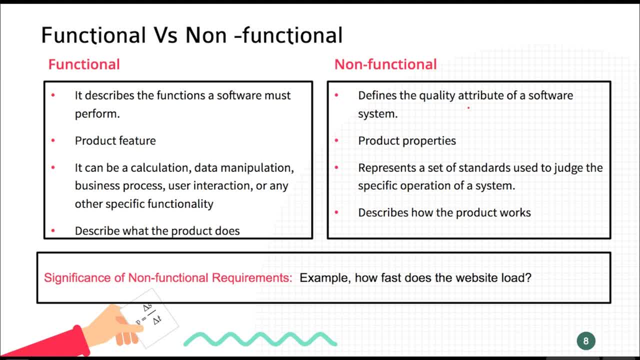 whereas the non-functional, it defines the quality attributes of the software system. The functional, it's a product feature, but you're so product properties. when I say functional, it could be anything: calculation, data manipulation or processing the user interaction. it could be anything, any functionality, the other 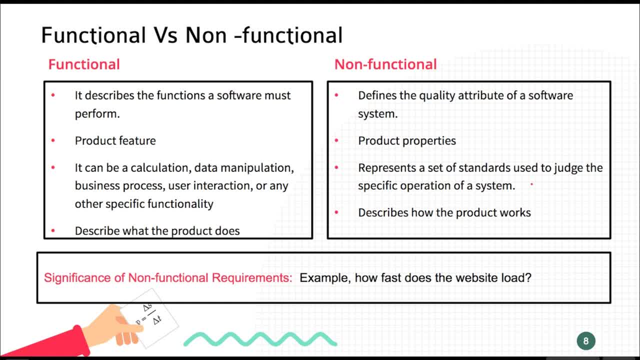 hand, the non functional is. it represents a set of standards used to judge the specific operation of the system. so, as mentioned earlier, when it comes to functional, it's described what the product does, when it comes to non-functional, how the product works right. so why do we need to have the non-functional requirements, is it? 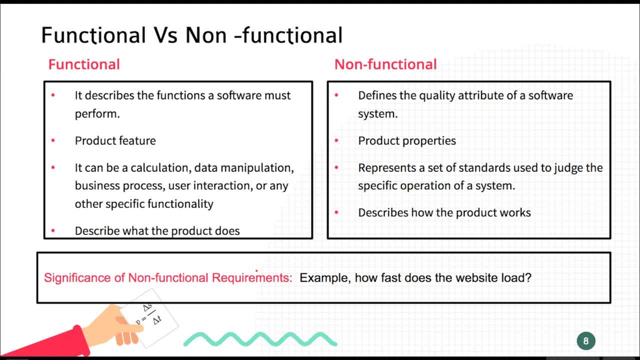 mandatory? no, it's optional. but it's a good idea to use non-functional requirements because it's a very, very important: the requirements which are not covered and the functional. it must be in the non-functional. so why do we need to use the non-functional requirements, right? for an example, how fast does the 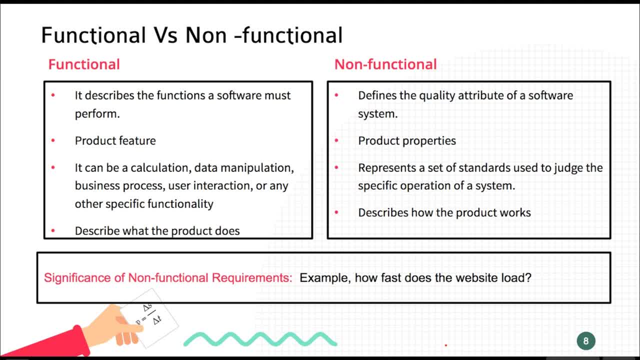 website load. let's assume you want to develop a mobile app, for example bank. when user logins with the login credential, it has to show the bank balance. now let's talk about the small use case. functionally, what is needed is: I want a mobile app. I have to open that. 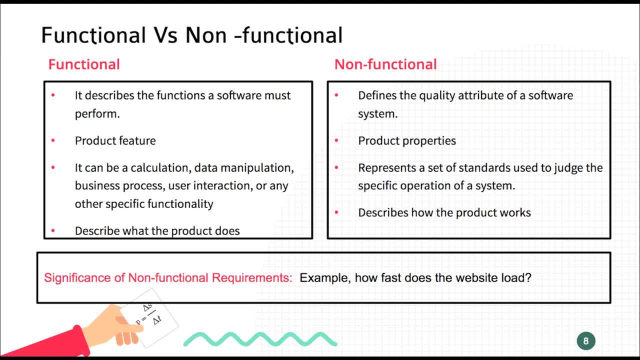 provide the credentials and it's going to populate the bank balance. that is a functional. let's see. I'll open up the app, I'll provide the credential. it takes like a five minutes to display the balance, even though functionally it works. but the quality is not there because, as a user, my 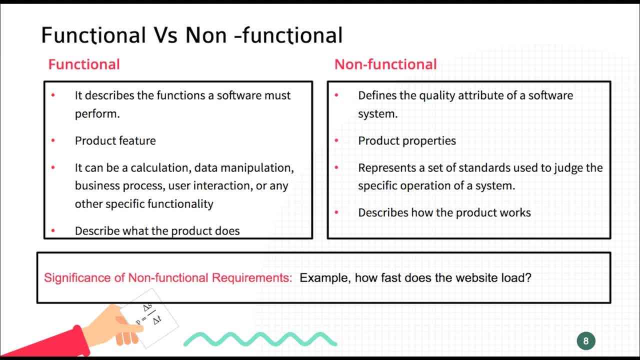 expectation is: I want to see my balance very quickly, as soon as I log in. it has to balance to be showed within, like you know, five seconds or 10 seconds max. but if the app takes like five minutes to display the balance, the functionality is there but the quality is not there. so, as the 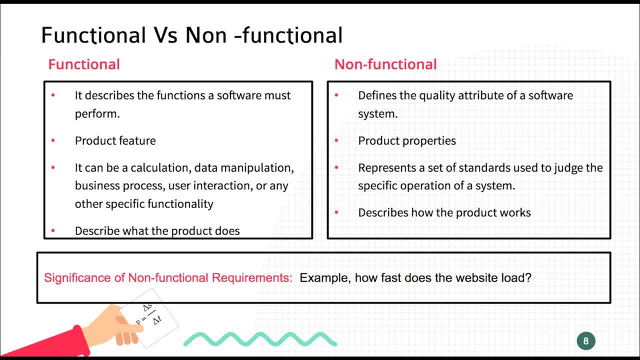 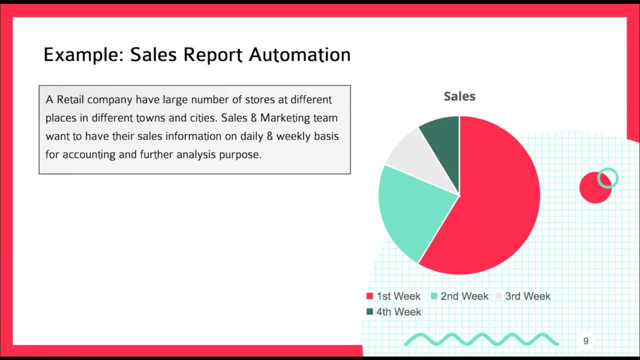 result: the bank is going to lose the customer base, right? so there is an example for a non-functional functional requirements and it's very, very important to define it in order to improve the quality of the software. so let's talk about an example in the sales report: automation. so retail company have a large number of stores at different 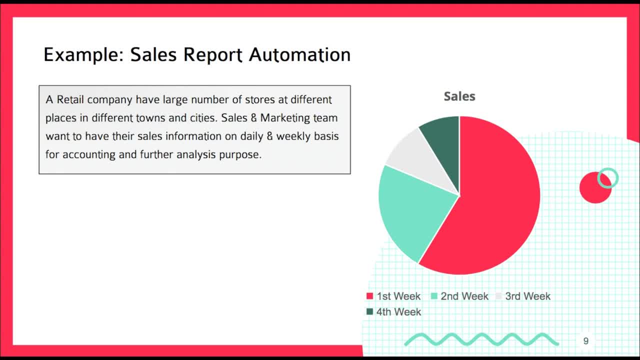 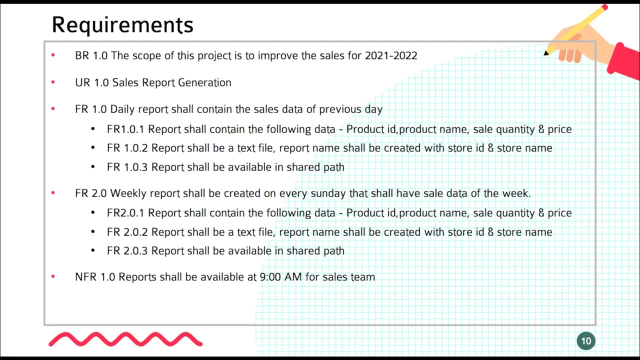 places in different towns and cities. okay, so the sales and marketing team want to have the sales information on daily and weekly basis for accounting and the further analysis. okay, this is the use case. let's see how the requirements are derived for this particular scenario. so what is the? 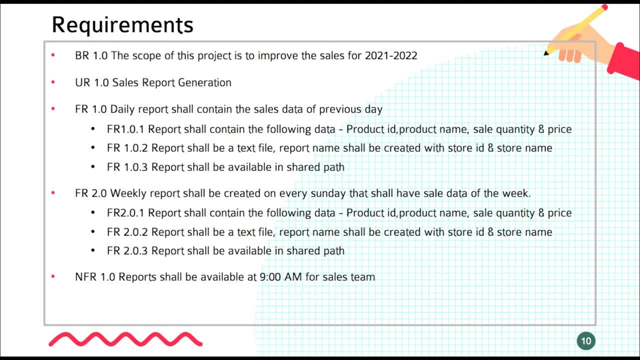 objective here. so we have to create a report from for the particular day or the weekly basis, right? so if you look at it here, I given the numbering. let's start with BR. that means it's a business requirement and UR is the user requirement, FR is the functional and the NFR is the non-functional. so business, 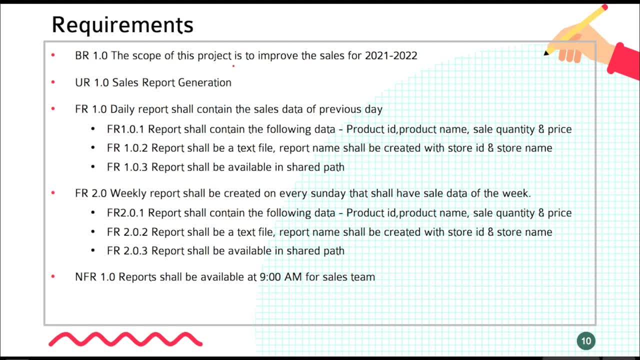 requirement is going to talk about the scope of the project to improve the sales for 2021 and 2022, and just for the discussion I'm bringing this and what is the user requirement? so who is the user here? the sales and marketing team is the users, so their equipment is to have the 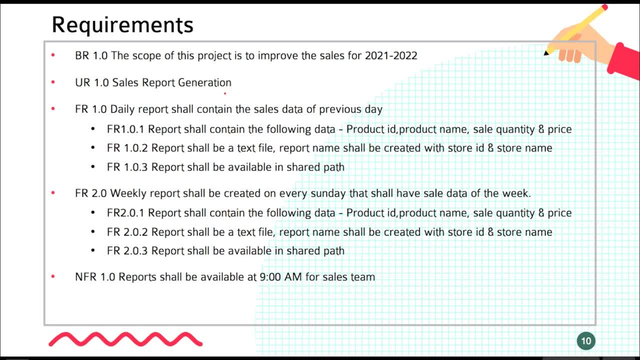 sales report. the user equipment does the sales report generation. by looking at this, the BR uh, the business requirement, or the user equipment development team cannot uh design or develop the, the requirement, the, the requirements. they want more information, right? what are the functions it has to perform? so those things would be covered in the functional. so the 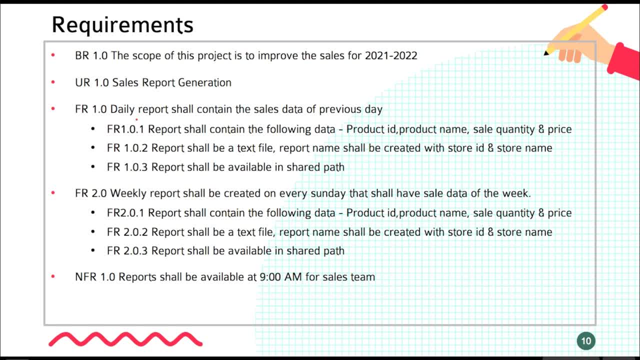 functional. it's going to talk about the daily report. daily report shall contain the sales data of the previous day and for the classification of the functional list, the report shall contain the following data. so I'm just giving example: the product ID, product name, sale quantity and price, and the report shall 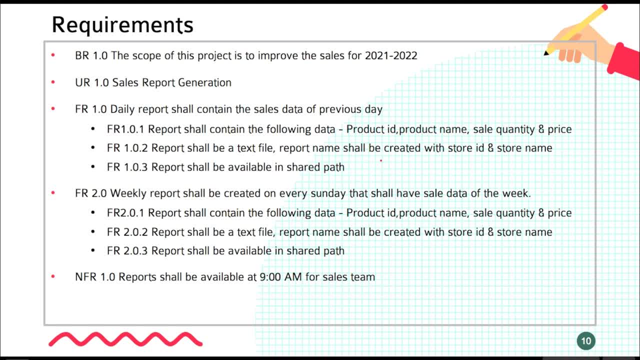 be a simple text file. a report name shall be created with store ID and the store name for identification purpose and report shall be available in the shared path for a team to access it. so this information is the base for development team and the testing team for development and testing it, even though they may not aware of. 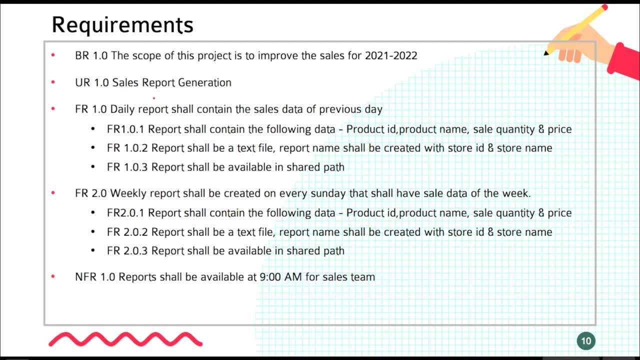 what is the scope of the business and what is the user recommend. by looking at the functional, as a developer, I'll come to know. I need to create a report. it's a daily report and what I? what are the information it should have and what is the name of the file and where should i place it. 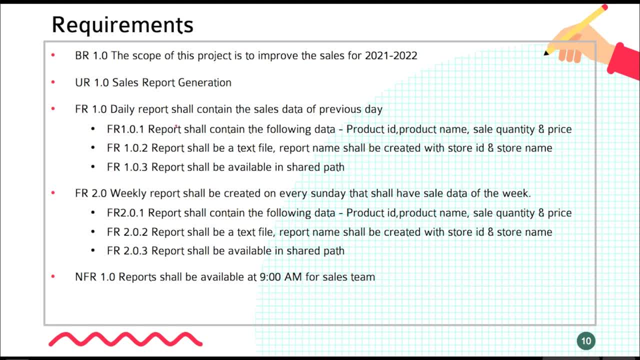 and this is the functional requirement of one. we are talking about the daily report, whereas the similar one we are going to do for the functional requirement 2.0 it's a weekly report. weekly report shall be created on every sunday that shall have sales data of the week. 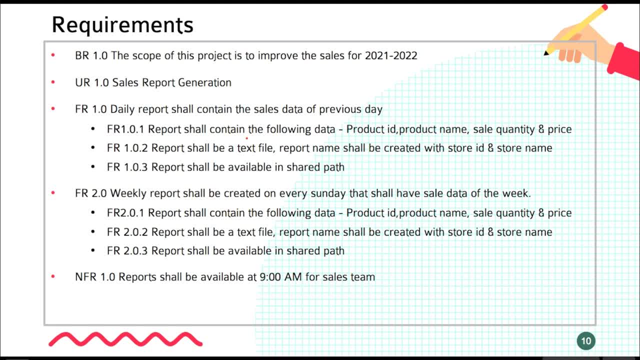 and it's going to have the similar as the daily. it's going to have the- the product id, name, sale quantity and price and the. it's going to be the tix file as daily report and, in order to identify, we should have the store id and the name as part of the file name. 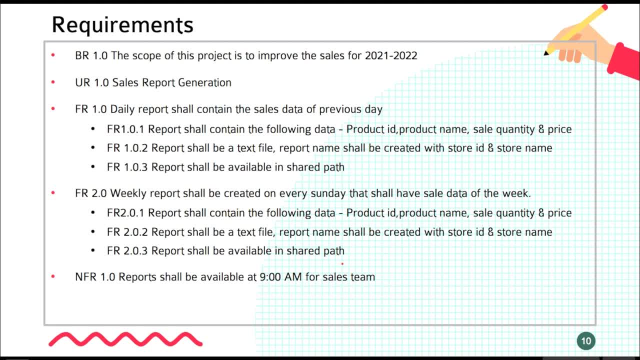 now, once the file is created, it should be there in the shared path. so by looking at this file, so we can see here that here we have the functional requirement one and two. that itself covered. what is the user expectation here? they want to create a report here.